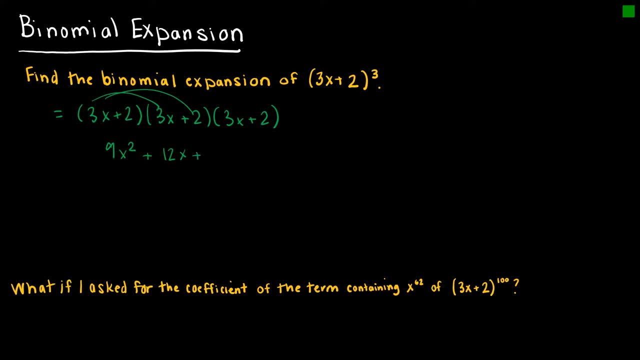 plus 6x plus 6x, so that's plus 12x, and then plus 4.. And I'm going to take that times 3x plus 2. And so I'm going to again just keep foiling. So I would get 27x to the third and then this: 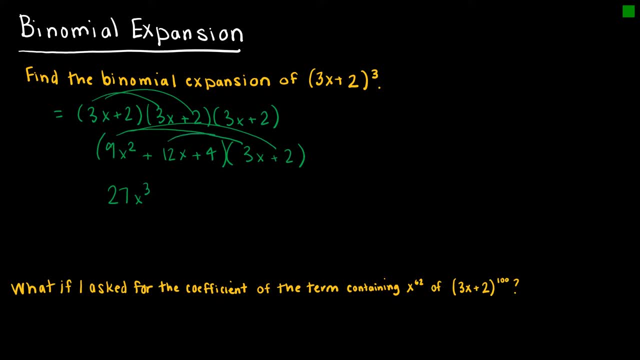 would give me 18x squared And this- I'm going to go ahead and write it out because otherwise I might make a mental mistake- 18x squared and then 12 times 3 would be 36x squared And then 12x. 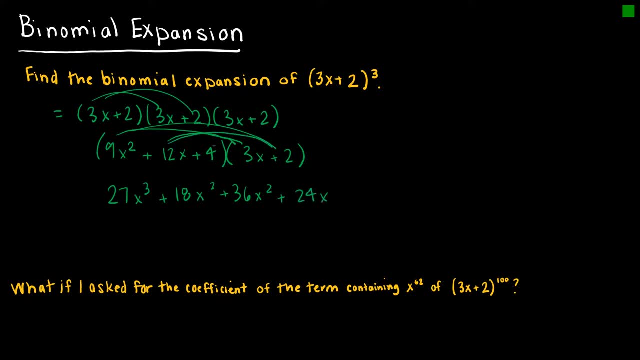 times 2 is 24x, and then 4 times 3x is 12x, and 4 times 2 is 8.. And so, if I simplify all of this, I have 27x To the third. I'm combining these together to get 54x squared. I'm combining these together. 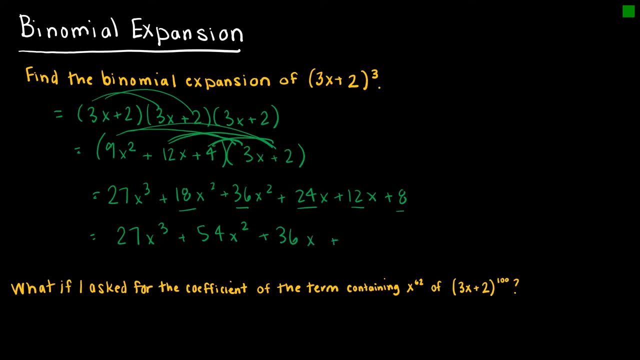 to get 36x, and then I have 8.. So that wasn't super horrible, and it's something we know how to do from long, long ago. But what if I said: hey, I want to know what the coefficient is? 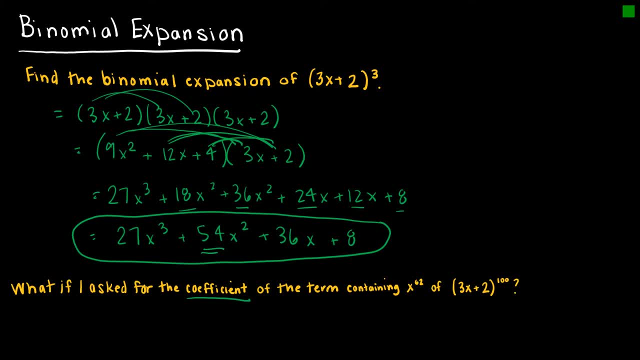 Remember coefficient's like: what's the number in front of the term containing x to the 16th? Let's add the number in and minus x to the 16th, So that's raise, end point, And you've got the diacritic. And now let's take return in and look at how thatじゃal. 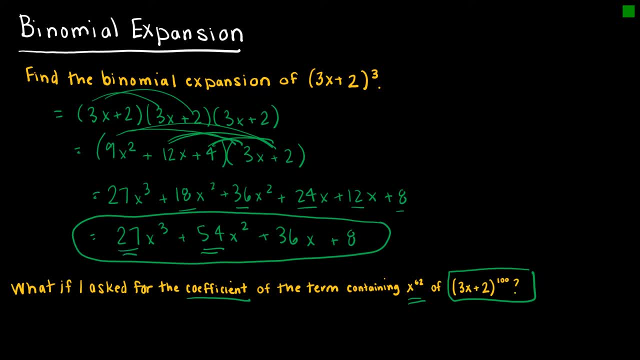 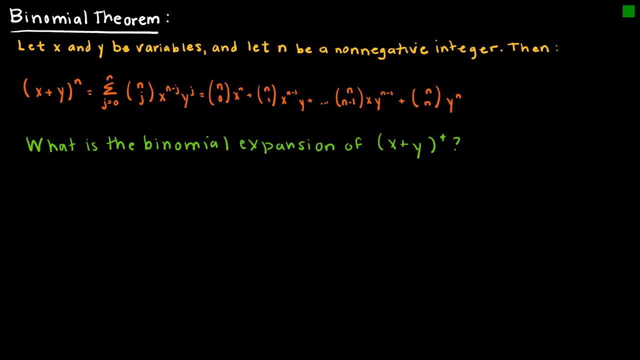 comes across. What if I again say I'm in on the declarations? and what if I write down my from 1 to 12th, and then in 2 to 16, and then in 3 and to the 16th, and then in 2 to 16 and 6?? 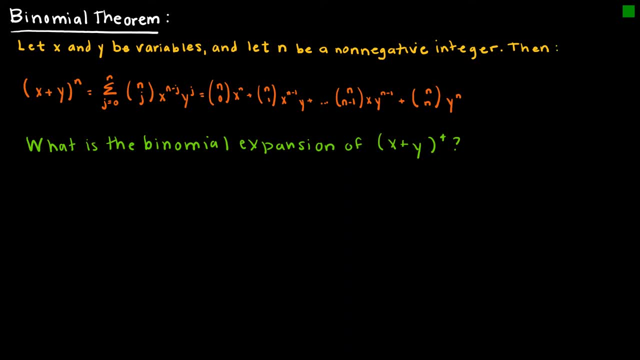 The expressionく will be 10x-2x-xx-2x-sx-eucin-x-al-time, Yes, t, and keep doing that over and over and over. so what we have here is we said we have the expansion of a and it's called a binomial theorem because again we've got two terms, x and y, and it could be 2x. 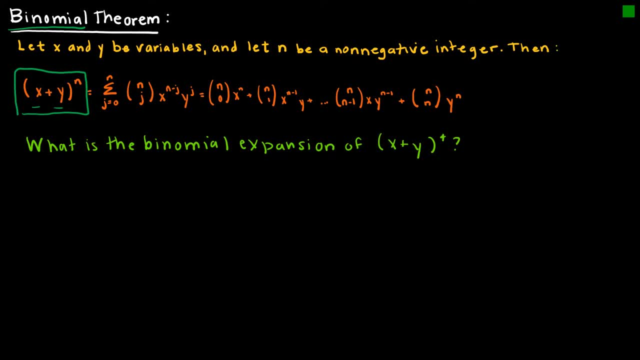 plus 7y, or it could be that y is just a constant. it really doesn't matter, it's the same pattern. essentially, what we're saying is we have the summation as j goes from 0 to n of n, choose j. so this is called a binomial coefficient, and that's really the goal here is to get those. 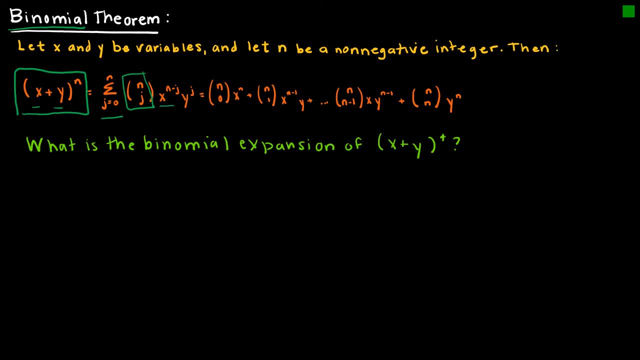 coefficients, and then x to the n minus j, y to the j, and so that might not make sense to you here. i've expanded it out for you a little bit, but to me it just makes more sense when i look at an actual example. so this one says: let's take x plus y to the fourth power, what would the binomial 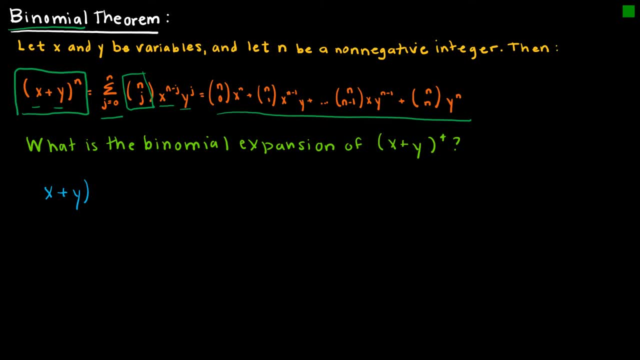 expansion be using this binomial theorem. well, it tells me that again i've got four because it's to the fourth, and i'm starting at j is zero. so four choose zero, and then i'm taking x to the four minus zero, which is four, and y is to the zero. 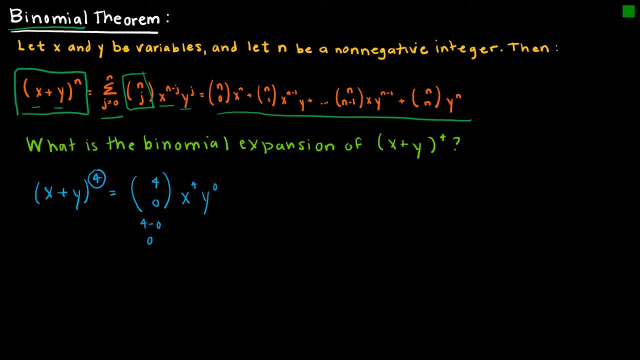 power. so y to the zero. now, typically, of course, i'm not going to write y to the zero. i'm doing it now just so you understand what's happening. then the next term is four. choose one, because it's going to increase. so as j goes from zero to n, so from zero to four, i'm going to keep going. 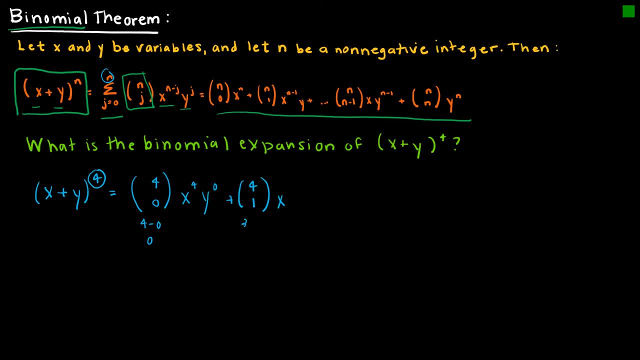 until i get to four, x is to the four minus one, which is three, y is to the one, and then four choose two. we can see the pattern here: x squared, y squared, four. choose three, x, one, y, three and four. choose four, x, zero, y, four. now, of course, as i said before, i'm probably not going to write this one, and i'm probably not. 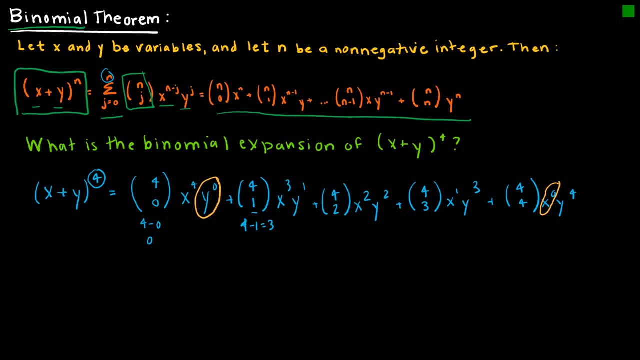 going to write this one in the future, because we already know what those are. but how does this really help us? because these four choose zeros are things that we already know how to do. four choose zero is the same as before, when i said four c zero or c four. 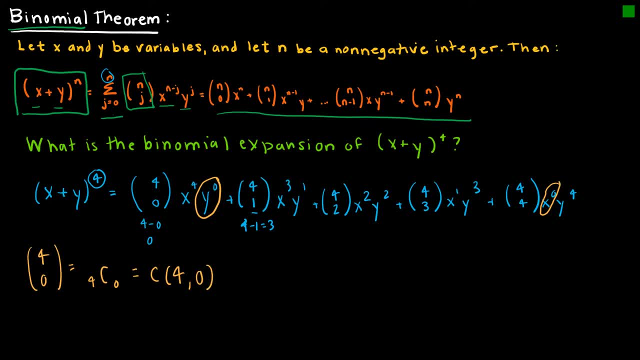 comma 0. All of those things are the same, And do I already know how to find that? That tells me to take 4 factorial over 0 factorial, 4 minus 0 factorial, and that ends up with 4 factorial over 4 factorial, which is just 1.. So this coefficient is 1. And I keep doing that for. 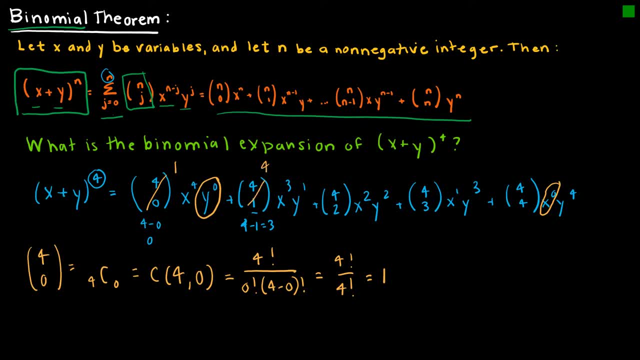 each of these. So 4 choose 1 is 4,, 4 choose 2 is 6,, 4 choose 3 is 4,, 4 choose 4 is 1.. And so what I have just found is that my answer to my expansion here is 1x to the fourth. 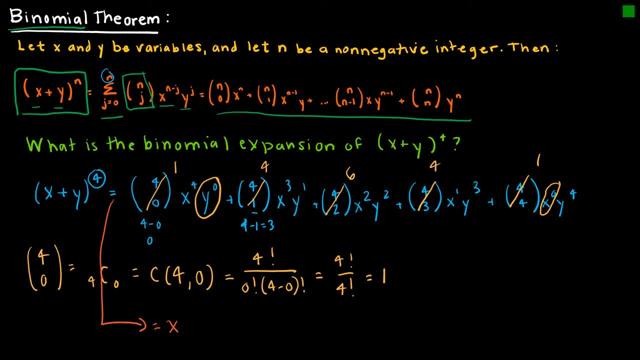 so I didn't even have to write the 1, but it's 1x to the fourth power and then 4x to the third, y to the first, and then six x squared, y squared, plus four xy cubed, plus again. I'm not going to write the one, I'm not going to write the X to the. 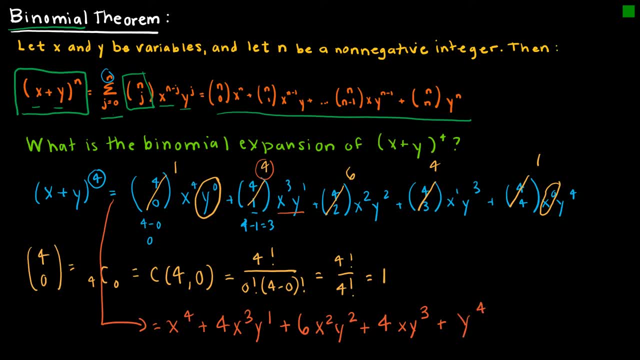 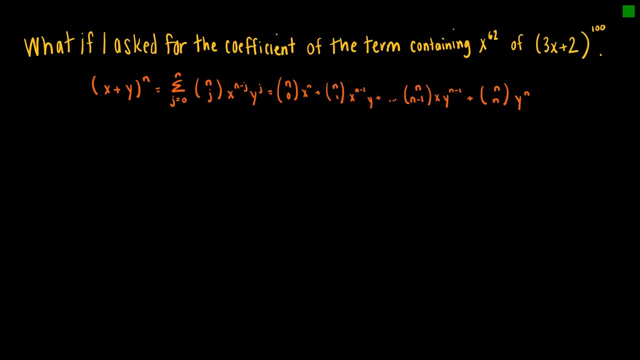 zero. so it's just y to the fourth. so I'm able to do the expansion of that without actually having to do any of the foiling. so let's go back to my original question that I didn't want to have to foil out by hand. what have I asked for? the 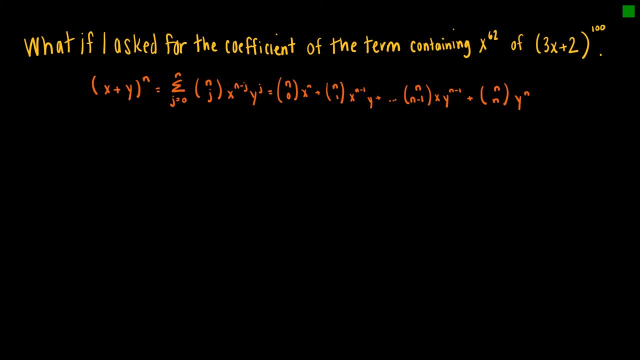 coefficient of the term containing X to the 62, of 3x plus 2 to the 100. so the first thing I should think about is again- and I've rewritten this binomial theorem for you, but it's okay to write this as the summation, and in fact I: 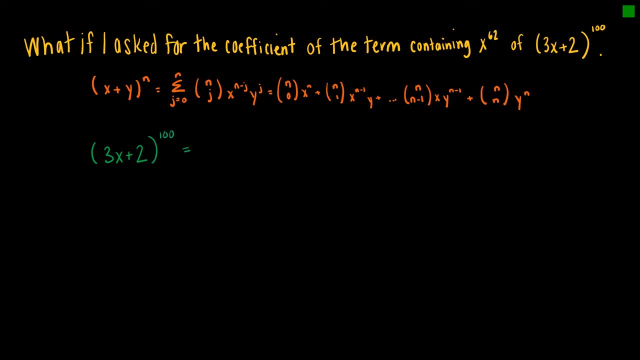 encourage you to write this as the summation and in fact I encourage you to write this as the summation and in fact I encourage you to because to me that helps it make sense when I'm trying to find a specific term. this tells me that I'm finding the summation as J goes from 0 to 100 of 100. choose J and again that. 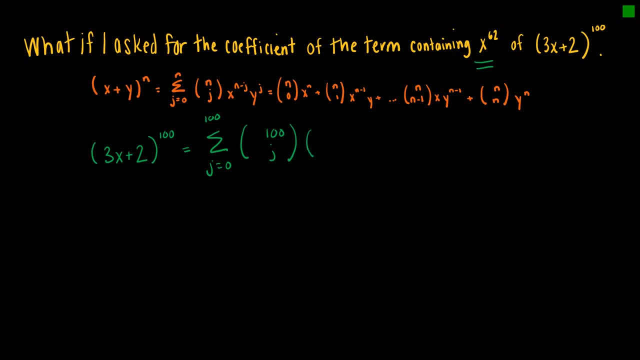 J is that value that is going to change, and then it's going to be, instead of just X to the N minus J, it's going to be 3x to the N minus J, so 100 minus J, because N is 100, obviously, and then instead of just Y to the J, I don't. 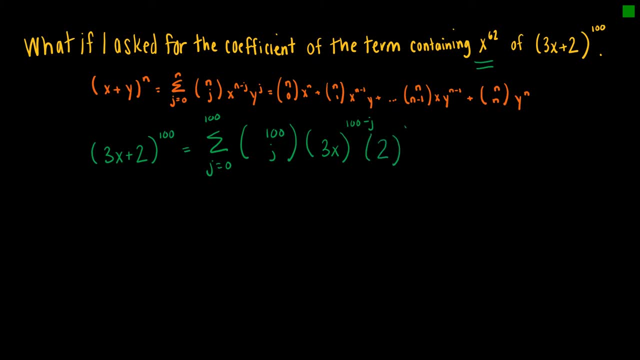 actually have a Y, it's just 2, and it's 2 to the J. so this is how I would rewrite it, using the binomial theorem as a summation. so what did that do for me? well, I'm trying to find the coefficient where X as a coefficient of 62, and so I 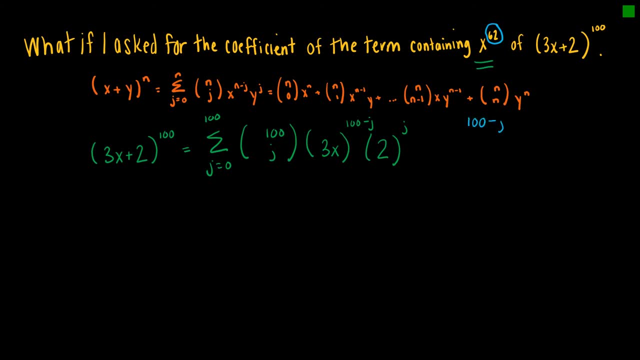 want to say that 100 minus J has to be 62. how do I know that? because I want X to have an exponent of 62 and this is the term with X on it. so 100 minus J must be 62, so J must be 38 again. now I'm going to take what I know here and I'm going 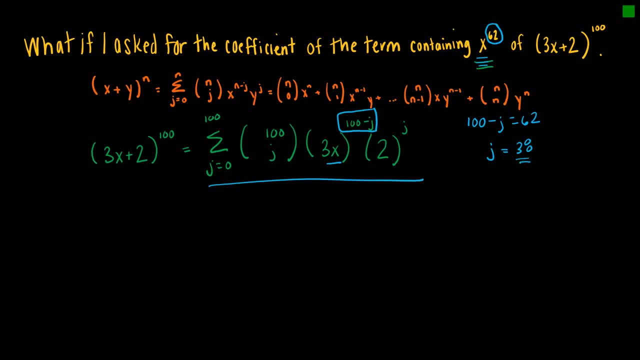 to use J of 38 to help me find the solution. So this tells me that the coefficient for x to the 62nd is 100 choose j, so 100 choose 68,, 3x to the 100 minus j, which was 62,, because that's what I 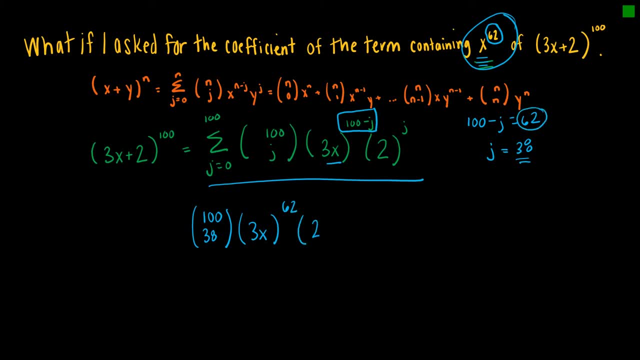 wanted right 62, and 2 to the j, which is 38. So that's going to be my solution, and now I just have to do the math. like I already have it set up correctly, This tells me I'm taking 100 factorial. 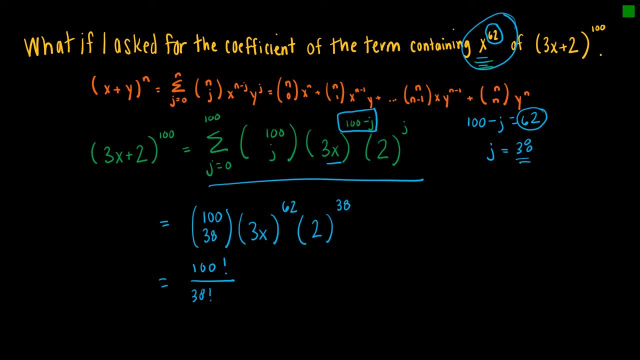 over 38 factorial, 62 factorial, and then this is obviously 3 to the 60, and this is 2 to the 38, and you might be asking: hold on, what happened to x? Do I really care about x? Well, I know that when I'm done, this is the number in front of x to the 62, but I'm really. 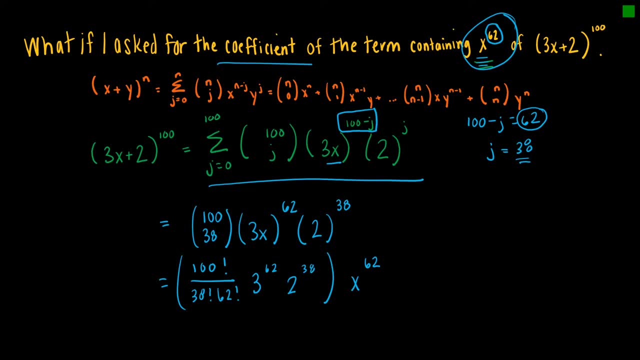 just looking for the coefficient, so I don't need to keep that x to the 62 on there. I'm just finding the coefficient. Now could I actually go ahead and compute this solution? I could, but this is going to be actually a little bit more difficult, So I'm going to go ahead and compute this solution. 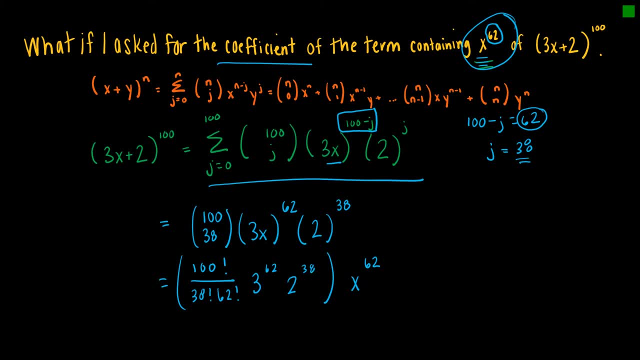 and I'm going to go ahead and compute this solution, and I'm going to go ahead and compute this solution astronomical. I mean, even just finding this value is. my calculator is not going to compute it because it's so many numbers that it just doesn't make sense. So again, as I had stated, 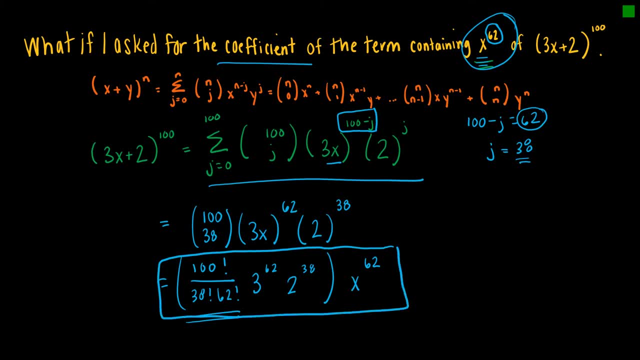 before. quite often in combinatorics, we just leave our answer in this kind of format, and so what would be the coefficient? It would be just this part right here. This would be my solution to that question. The last thing I want to talk to you about this week is: 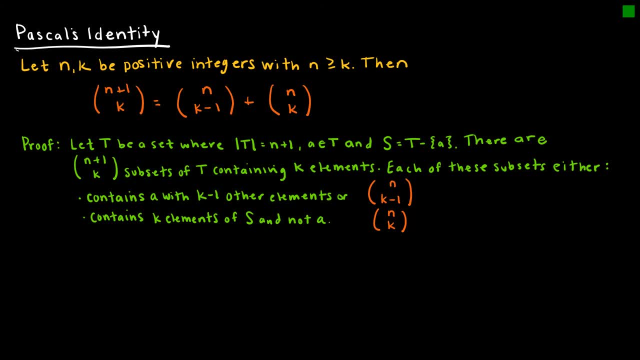 Pascal's identity and Pascal's triangle, which are obviously related. And Pascal's identity says: if n and k are positive integers with n greater than or equal to k, then n plus 1- choose k is equal to n. choose k. minus 1 plus n: choose k. And again, this is just an identity that you're going. 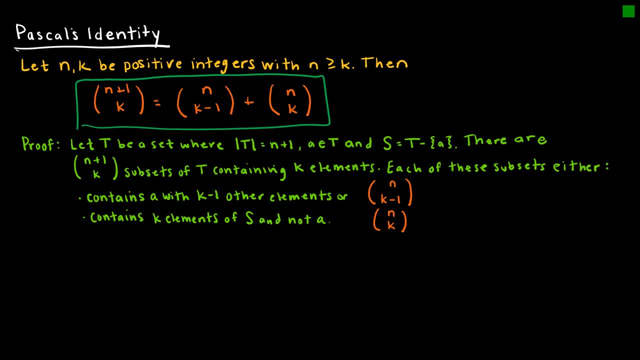 to use literally all of the time in combinatorics. We're going to use it, you'll need to know it. But for now again, it's just a nice, nice introduction, And I've included the proof here so you can kind of see or understand why. 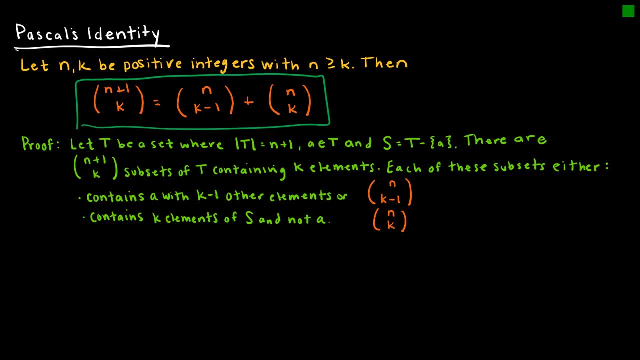 this identity works. So we're going to say: let t be a set where the number of elements in the set of t is n plus 1.. So we have n plus 1 elements And a is in the set t and s is t minus the element a. 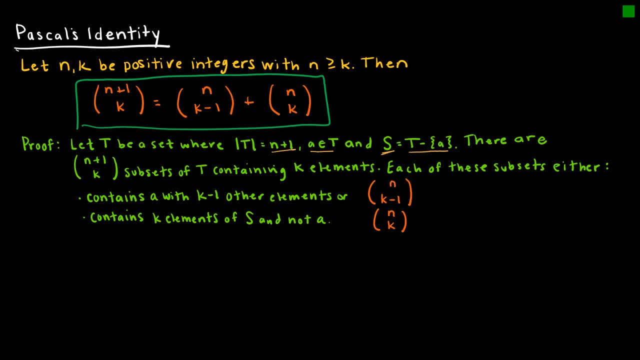 So essentially we're saying there are n plus 1, choose k subsets of t that contain k elements And each of those subsets- either- so this is equal to- either contains a with k minus 1 other elements, or it doesn't contain a and therefore there's k elements in. 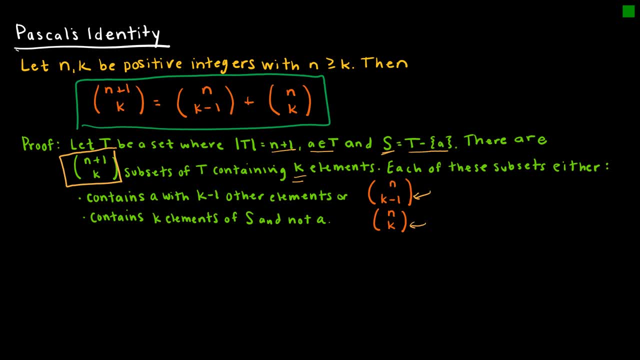 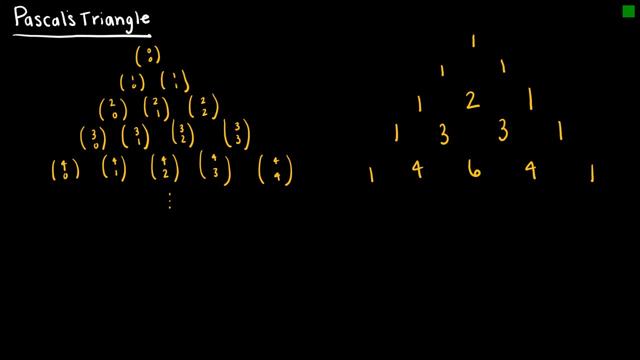 there. So that's just a way to show that the two sides are equal to one another. So why does this matter? Well, because Pascal's triangle is based on that identity. And Pascal's triangle, if you can see this, is just zero, choose zero, and then one choose zero, and then one choose one. 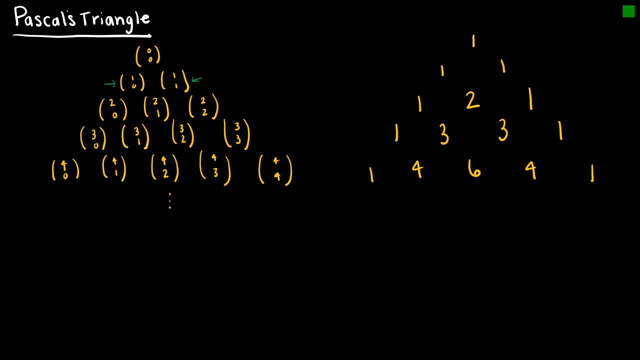 and then two choose zero, two choose one, two choose two. These are the rows of Pascal's triangle. Well, what does that do? for me, Pascal's triangle is, if you'll remember, we worked through x plus y to the fourth And we found the coefficients we. we did all of this using 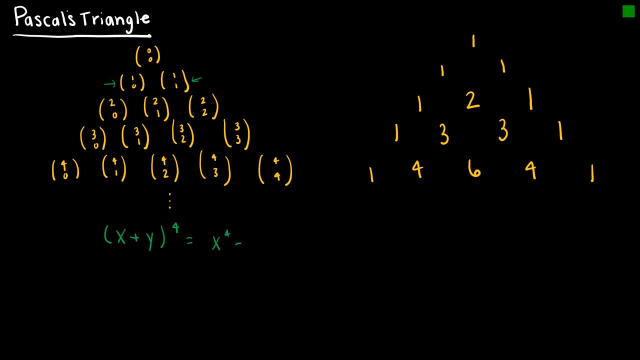 the binomial theorem And we said that was x to the fourth plus four, x to the third, y plus six, x squared, y squared plus four, x, y cubed, plus y to the fourth. So we just did this together a. 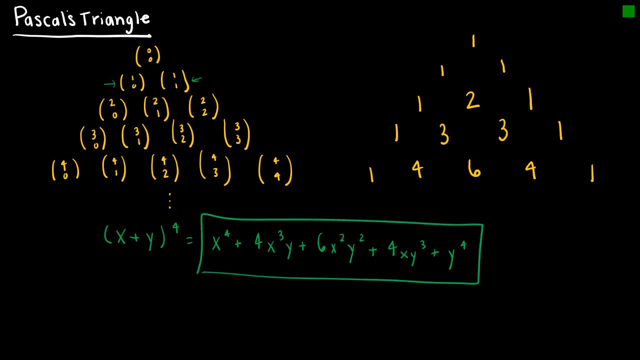 little while ago. So Pascal's triangle says, hey, those numbers one and four and six and four and one can be found And in this row of Pascal's triangle one and four and six and four and one. So why does Pascal's 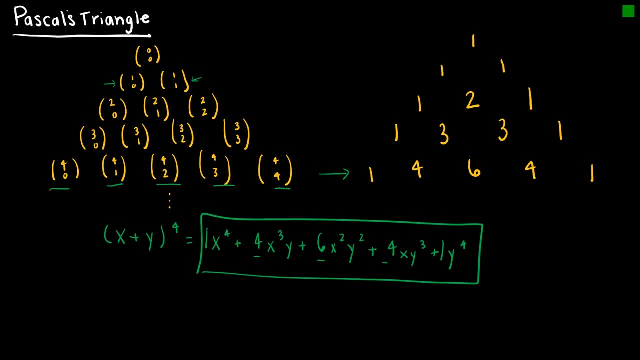 identity matter. then Where does that come from? Well, Pascal's identity says: if you've got two consecutive elements, you can add those together to get the next value of your Pascal's triangle. So three plus three is six, and one plus three is four, And you get the idea And I can make the 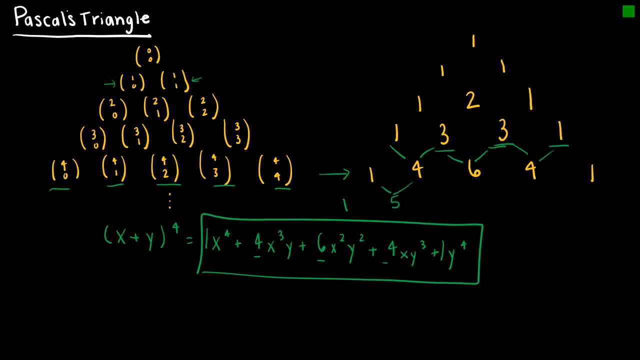 next row as well. This would be one. One plus four is five, Four plus six is ten, Six plus four is ten. Four plus one is five, And then one, And so this would be the next row of Pascal's triangle. So we can see how that might be nice. 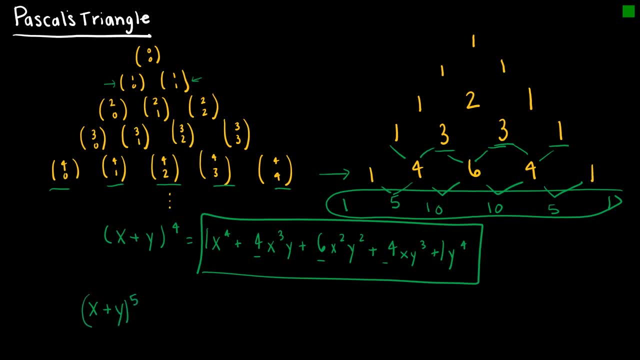 If I wanted to take x plus y to the fifth, then I can easily say: well, that must be one x to the fifth plus five x to the fourth, y plus 10 x to the fifth, And that's the second row of Pascal's. 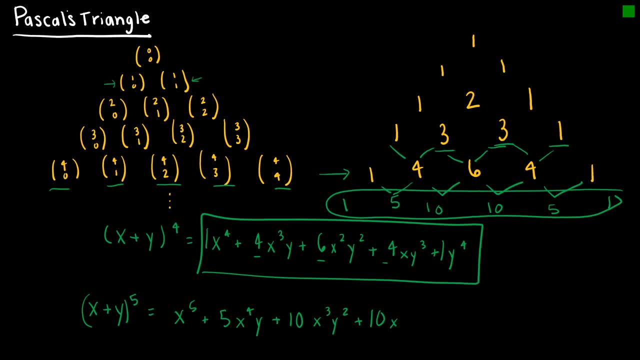 the third, y squared, plus 10 x squared, y to the third, plus five x y to the fourth plus y to the fifth, And I didn't have to do any work. I just looked at Pascal's triangle and really just cheated using Pascal's identity. So that is where Pascal's triangle comes in, very helpful.